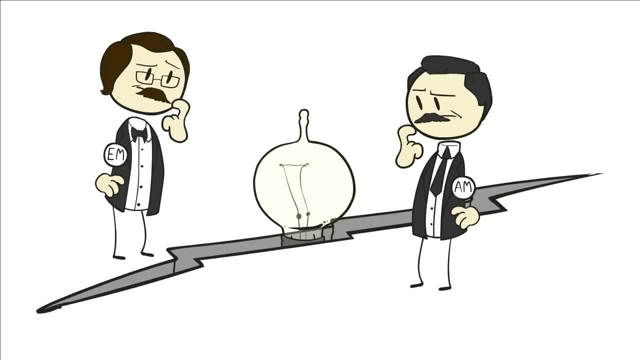 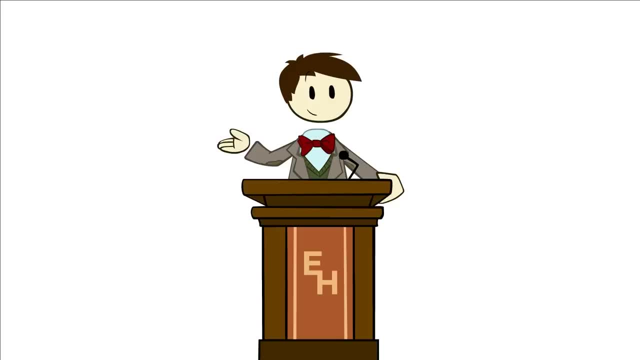 See, this was the central mystery stuck in the craw of physics By the end of the 19th century. this problem of how light moves was becoming impossible to ignore Because, at the time, light was largely assumed to be a wave, just like sound or waves of water. 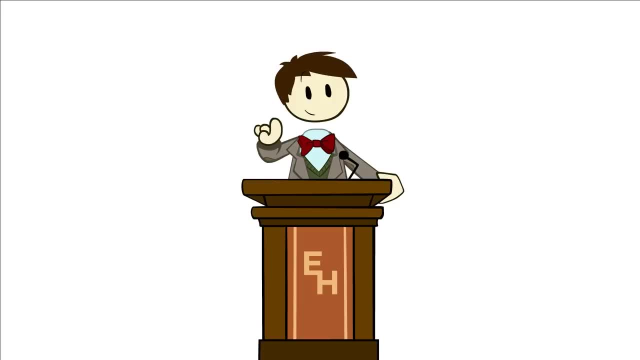 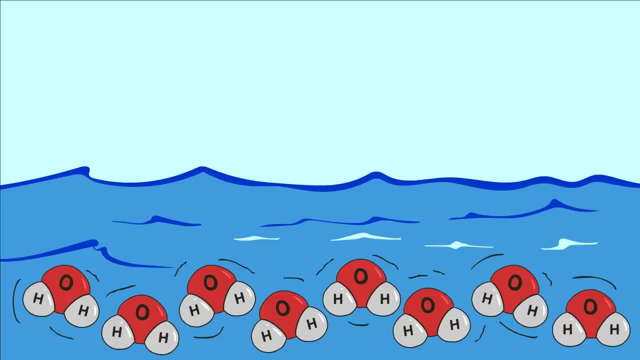 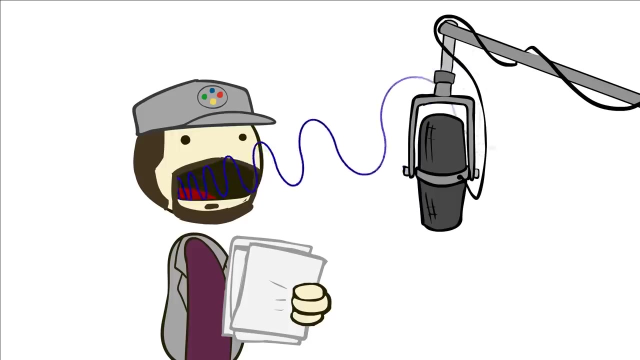 But the thing about those types of waves is that they have to travel through stuff. A wave is just a motion, and to have motion you have to have something being moved. Waves of water are simply motion, propagated through the molecules of water. Waves of sound work the same way, traveling by rippling through the air. 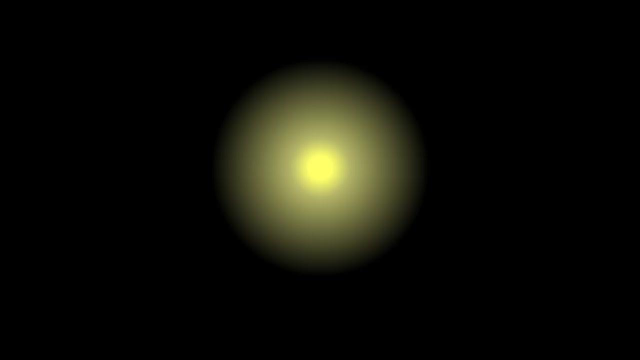 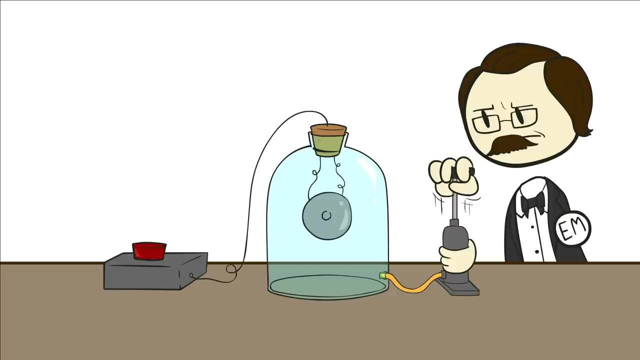 But light travels through a vacuum, and that's a problem. Experiment after experiment had been done, where a complete vacuum was created, where all the air and other matter was pumped out of a container and then waves were pushed through, Sound died. 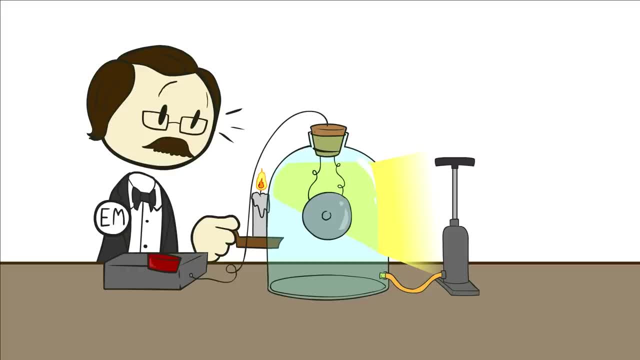 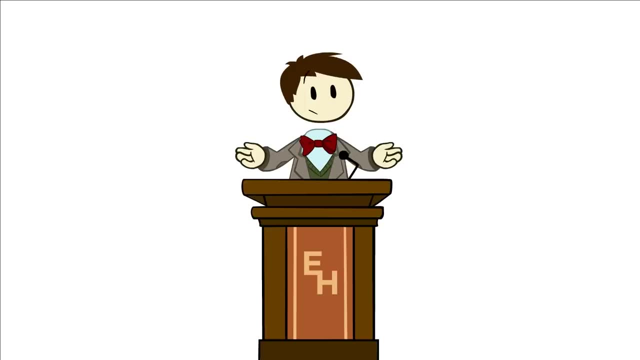 The wave couldn't travel through nothing But light. Light traveled across the void. How did it do that? The theory at the time was that there was some giant invisible, incompressible fluid that permeated all things. They called it the ether. 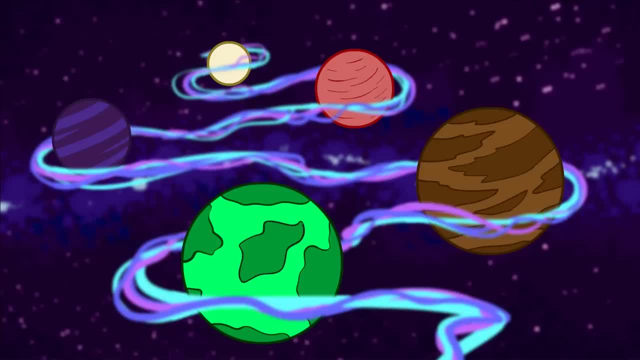 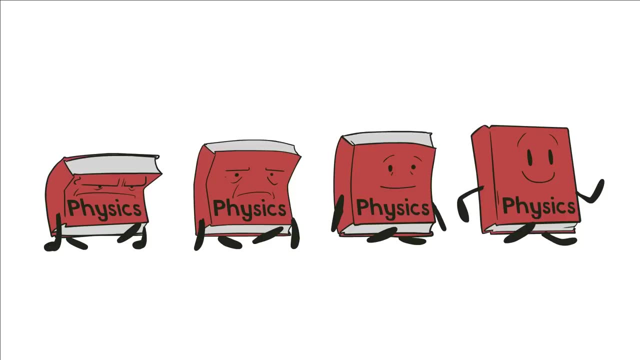 It filled the dark between the stars and subsumed the void between worlds, And it was through this fluid that waves of light moved. The only problem was that, well, as physics got more and more advanced, we started to have to assign wilder and wilder properties to this ether. 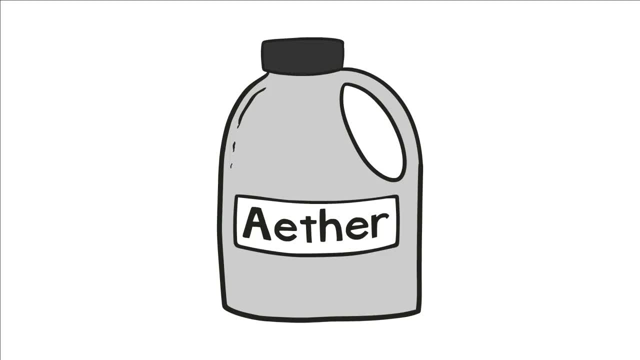 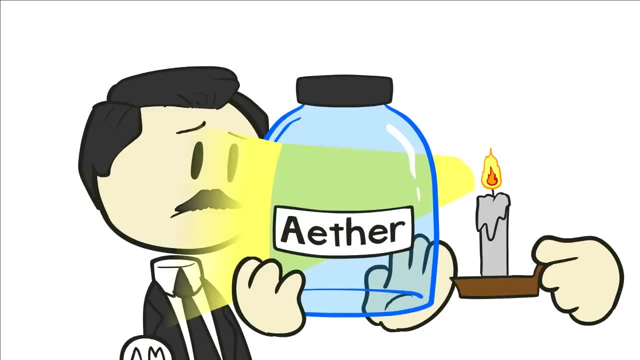 It had to be fluid but totally rigid also, And it had to be incompressible but also totally massless. It had to be utterly transparent and yet also be a medium for light. Still, there was no better explanation, so, even as serious questions were raised, 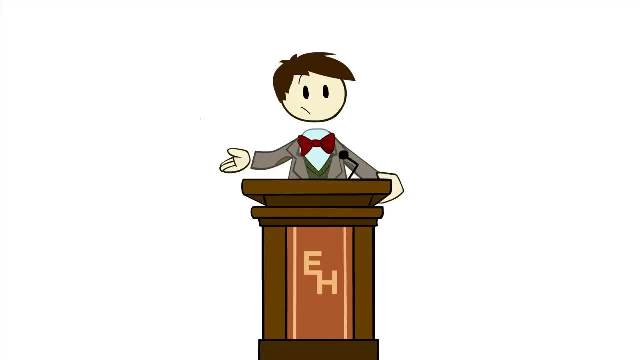 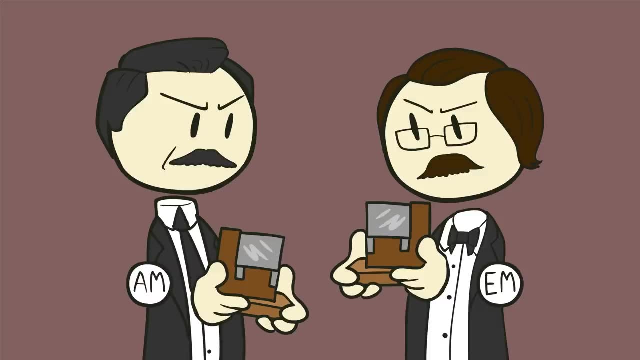 the idea of the ether served as the working theorem for most of the scientific world, But as the 19th century began to draw to a close, people were finally starting to figure out ways to build a contraption sensitive enough to test for the ether. 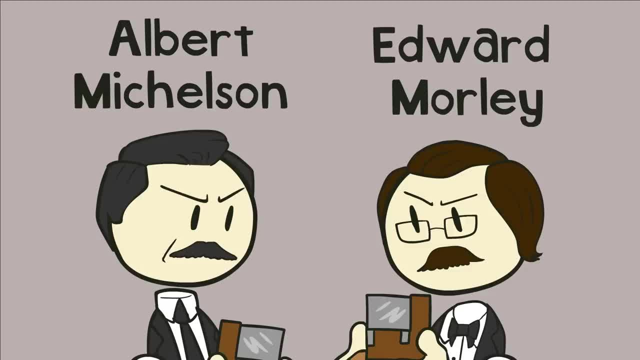 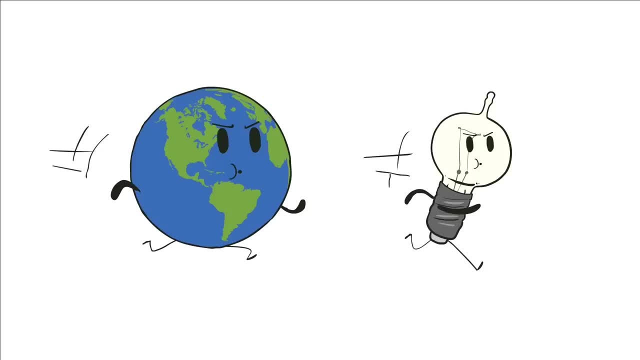 Those people were Mickelson and Morley. They had created a device so precise that it should be able to detect the effect of the speed of Earth on the speed of light. What does this mean? Well, imagine that you've got two sets of people playing catch. 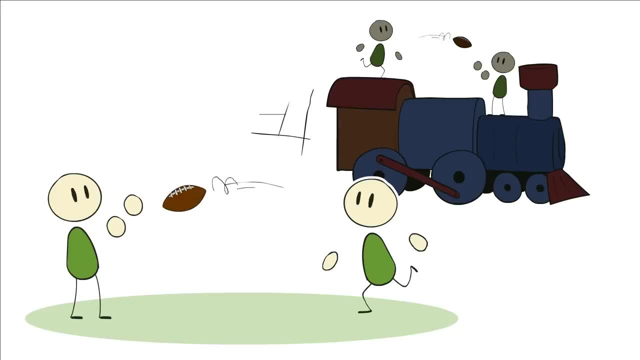 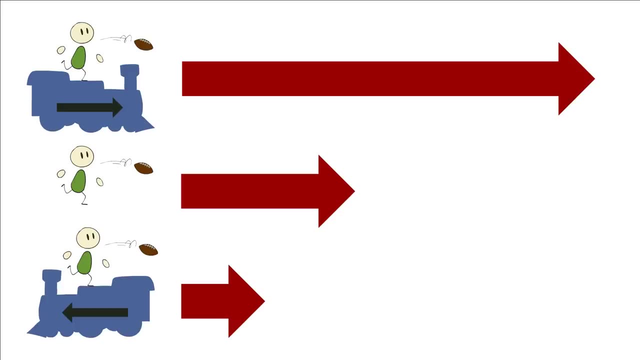 One set of people are on a moving train. one set of people are on the ground next to the train. They both throw the ball at the same speed, but relative to the people on the ground, the ball thrown on the train either moves much faster or much slower. 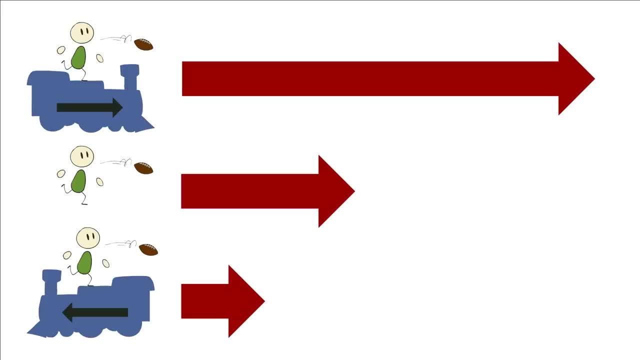 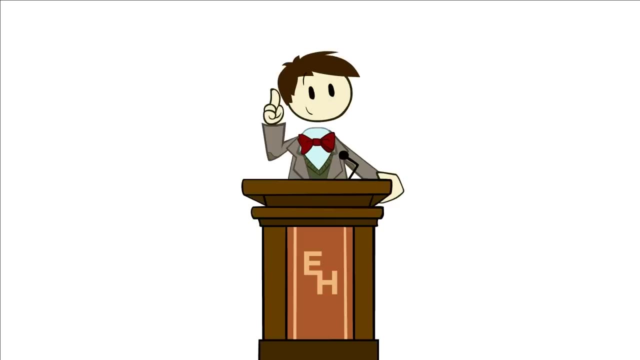 depending on whether it was thrown with or against the motion of the train. By this point in history, we had already worked out a speed for light against the fixed reference of the ether, which, in our previous analogy, is basically like the people on the ground throwing the ball. 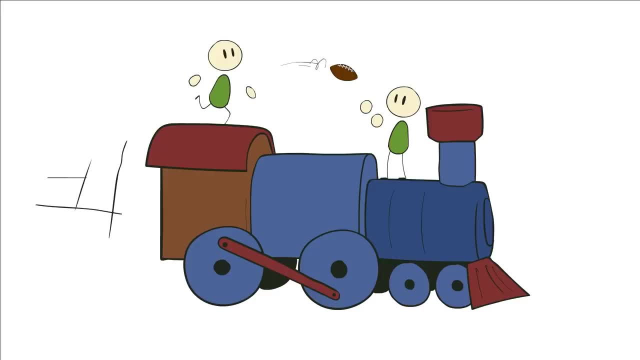 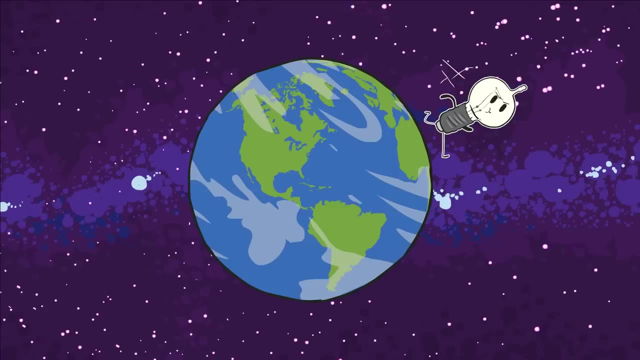 What Mickelson and Morley set out to do was work out a method to figure out the case for the people on the train. How did being on the planet Earth, hurtling through space, affect the speed of light? Unfortunately, the Earth doesn't move very fast compared to the speed of light. 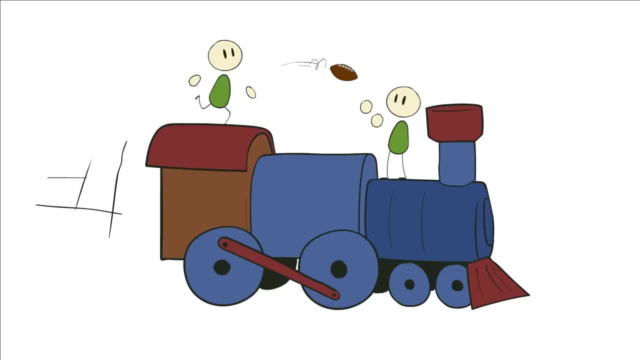 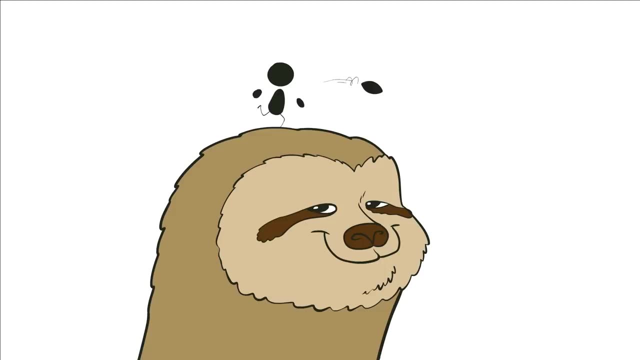 which made this a pretty challenging thing to test. Instead of throwing a ball on top of a train, this was sort of like trying to measure the effect of throwing a ball from on top of the world's biggest, slowest sloth. Hence them burying the experiment underground, resting it on mercury. 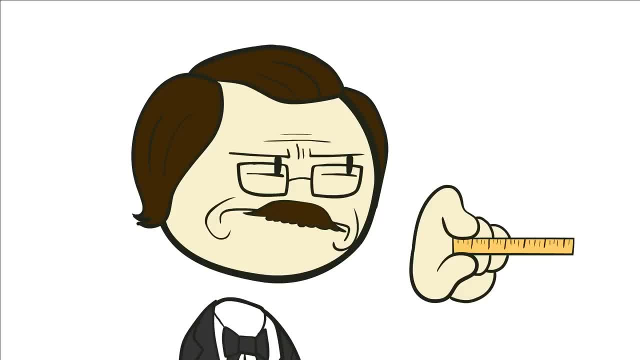 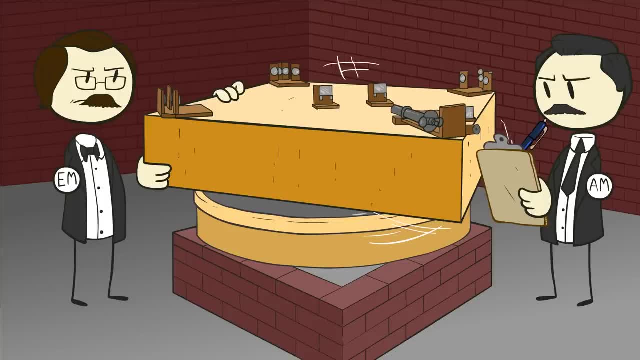 and placing limestone on that mercury. They would need to test it. They would need to measure something so small. they couldn't have any wayward trimmers messing up their results, even as they adjusted their experiment and spun it around. But- and this is one of the triumphs of experimental physics- 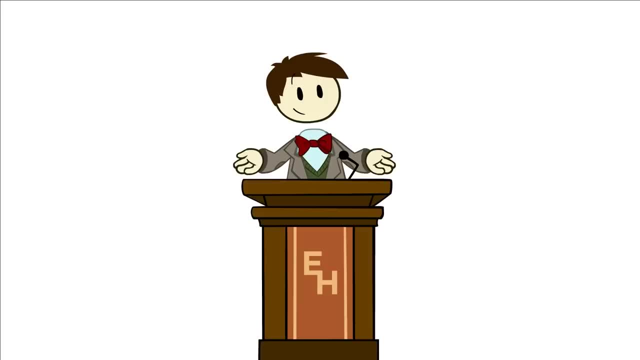 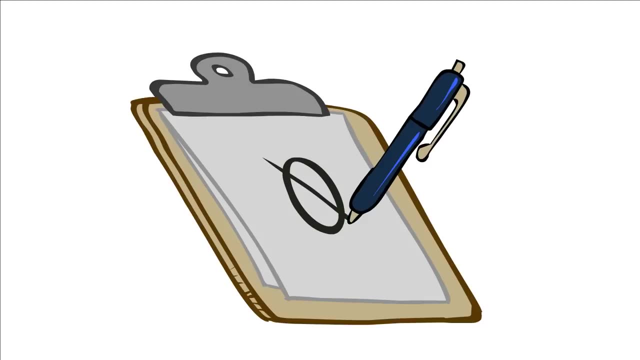 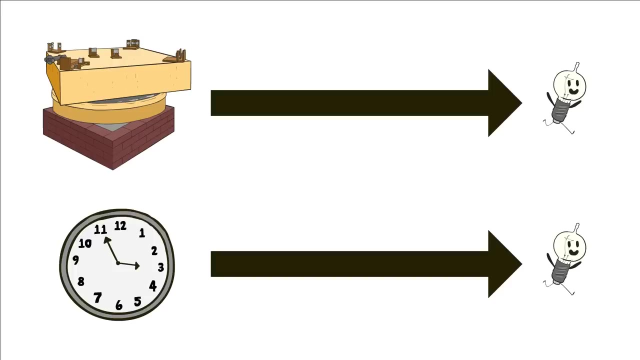 they did it. Their experiment was so exact that it was hard to dispute that it should be able to pick up the effects of the ether wind. Only it didn't. There was none. They got no effect at all. Light moved at the same speed, no matter how they turned their device. 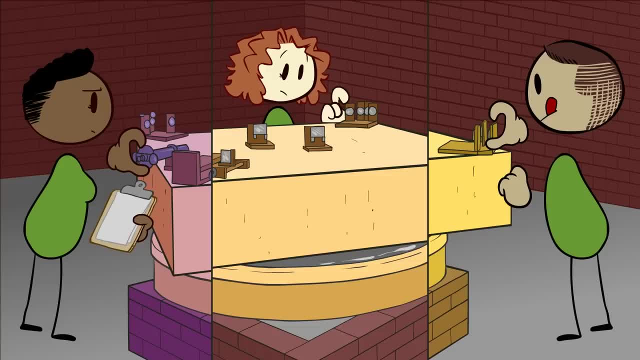 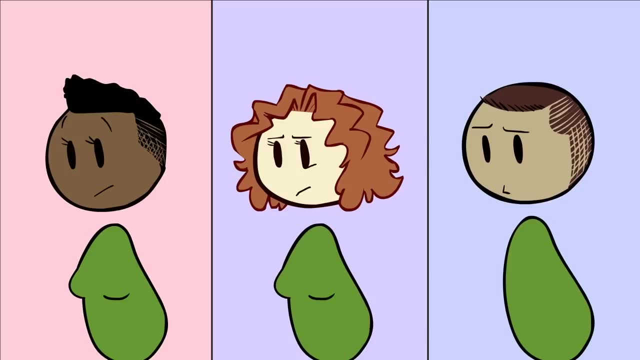 no matter when they took their readings. It was astonishing. Countless times people would try to refine this experiment, hoping for a different result, And countless times it would just confirm There was no ether. Ether was not a thing. This threw science into chaos. 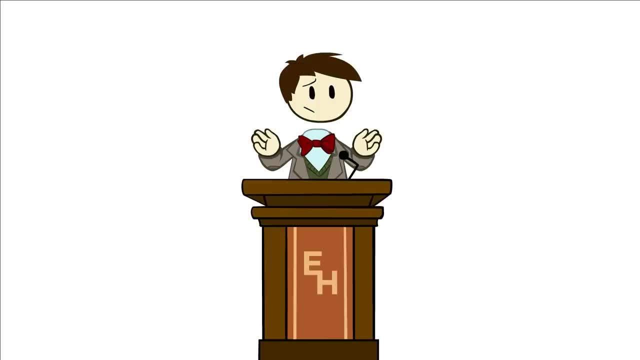 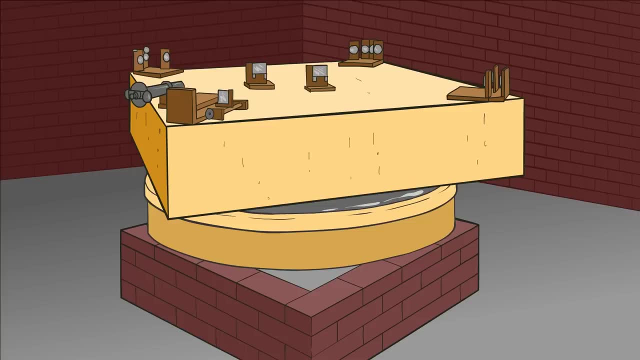 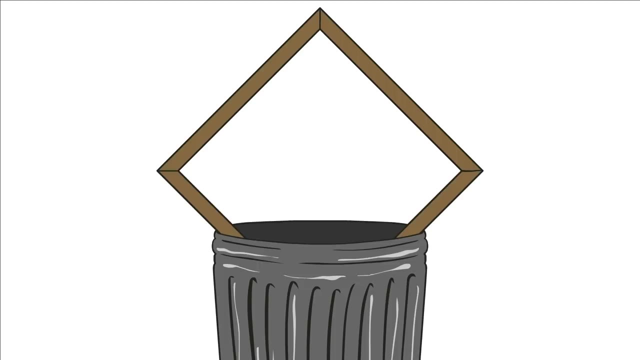 What could the explanation possibly be? How could we make sense of this? Well, in 1905, a young man named Einstein would propose a solution Inspired by the Michelson-Morley experiments. he would offer us special relativity, which is called relativity because it does away with the concept of an absolute frame of reference in physics. 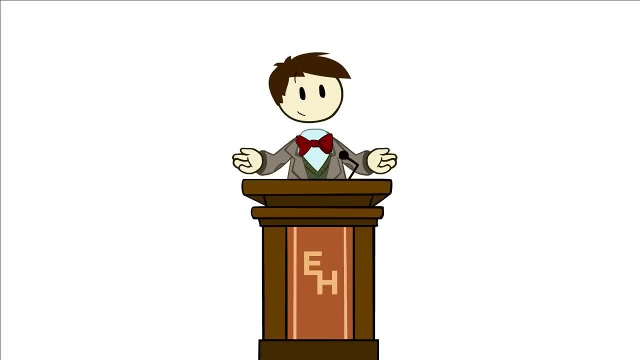 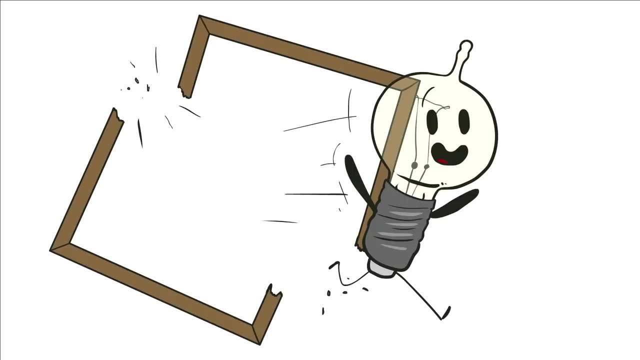 By which I mean the ether. This led to a number of other conclusions, such as proposing that the speed of light in a vacuum was constant, that it wasn't actually affected by frame of reference, and that we would have to see space and time as one contiguous thing. 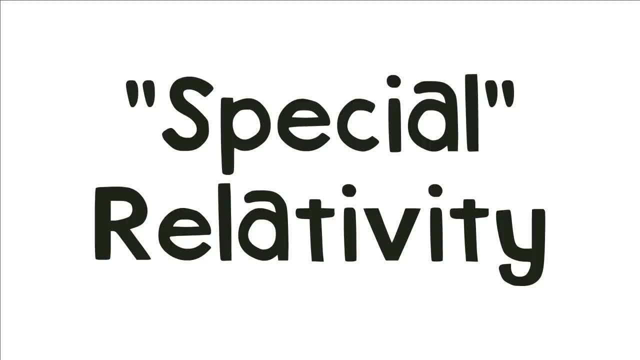 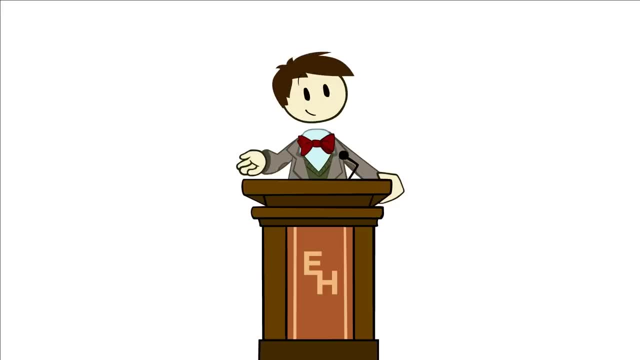 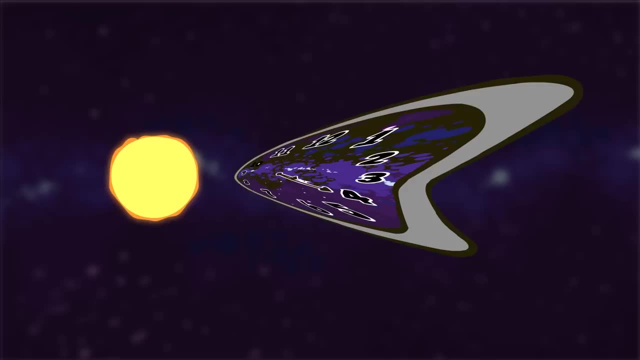 rather than two completely separate ideas, But it's called special relativity for a reason. This paper pointed to something else, something even stranger than the idea that space and time were one, And that was the idea that space-time might be curved and that the curvature of space-time 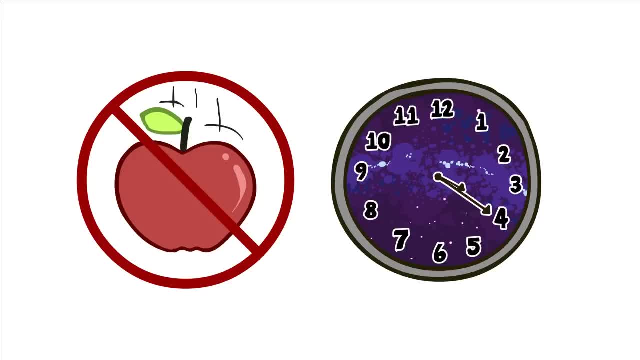 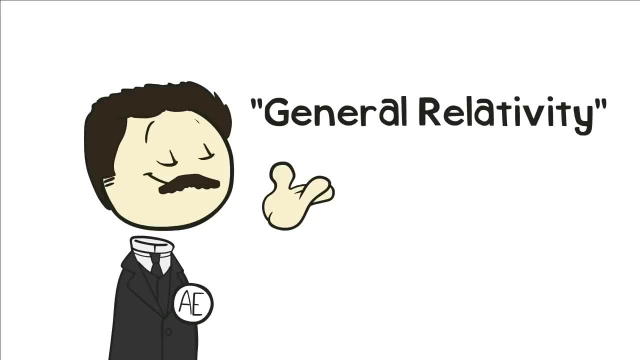 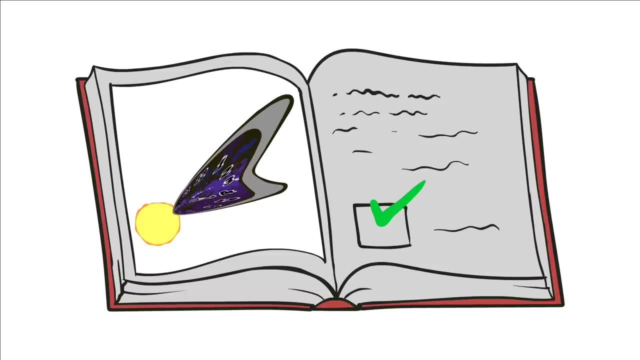 might be affected by gravity. The special version of relativity only dealt with physics where gravitational distortion wasn't really present, But in 1915, Einstein would give the world the far more complex theory of general relativity, One that was applicable even where stars or black holes bent. 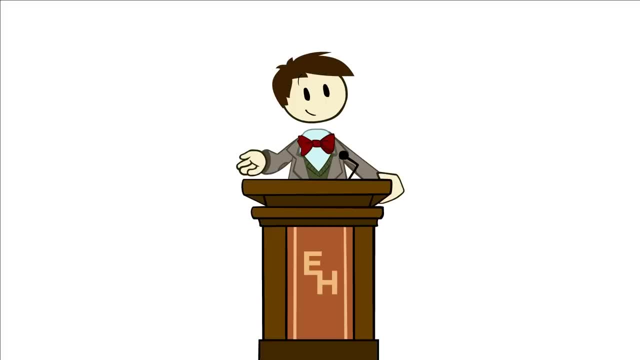 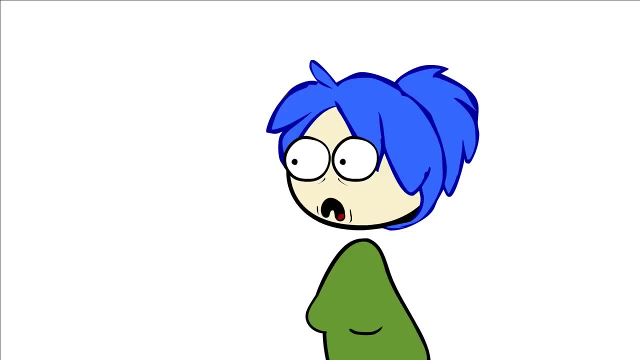 and warped the fabric of space-time, And it's that curvature of space-time and the way those curves get warped and changed that we are interested in here in this series, Because one of the most frightening things about accepting this new way of thinking, of accepting relativity, is that it also 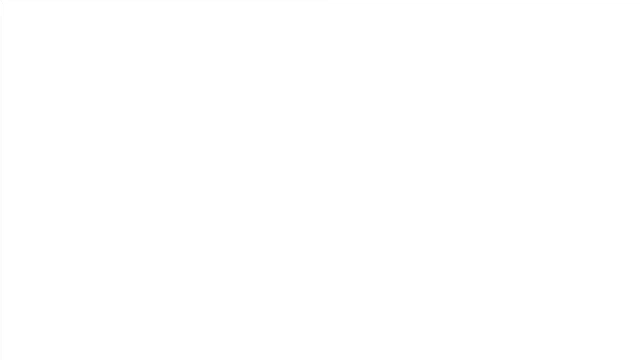 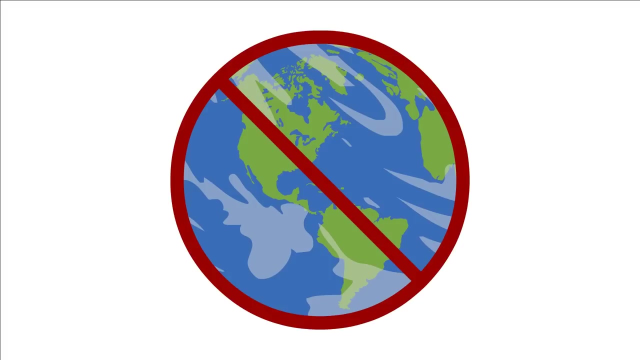 means that we have to accept that we live in a non-Euclidean universe. Postulate 5 really isn't true in any higher sense. It doesn't represent the world as it actually is, In fact, the strange geometries of Galilei, Lobachevsky and Riemann. 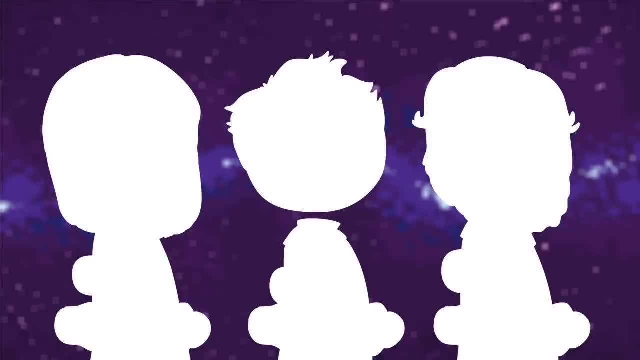 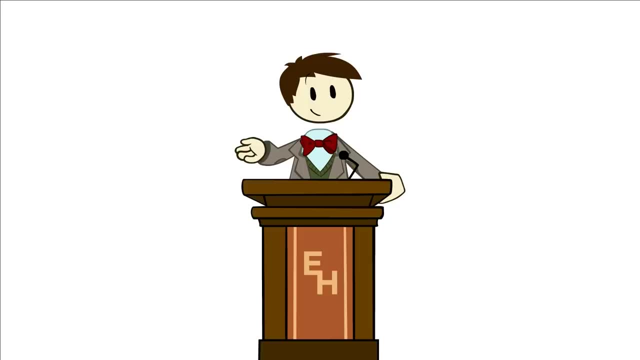 were much closer to the truth. They are a far more accurate representation of the universe as we now understand it, And it is those geometries that we now use for much of modern physics. So the geometry that we built all of mathematics, on that we 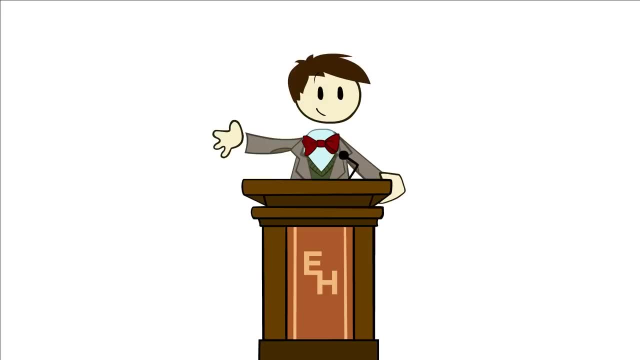 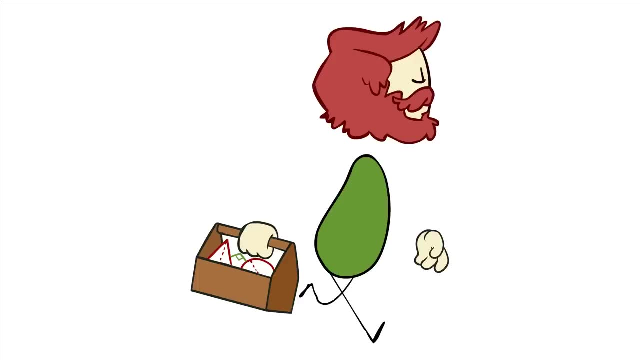 built all of our calculus and our Cartesian coordinate system out of that gave us Newtonian physics. in the end, it wasn't in any way real. It was and is simply a useful tool created by humankind. It was a way of thinking and 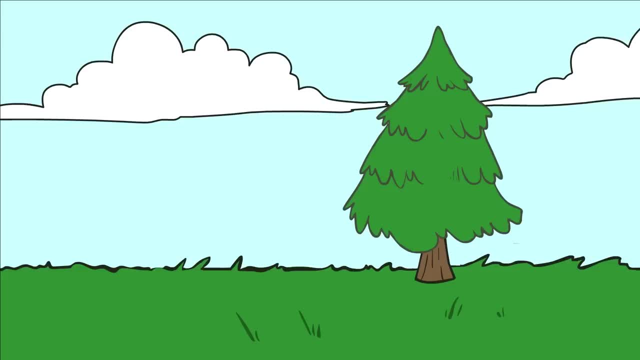 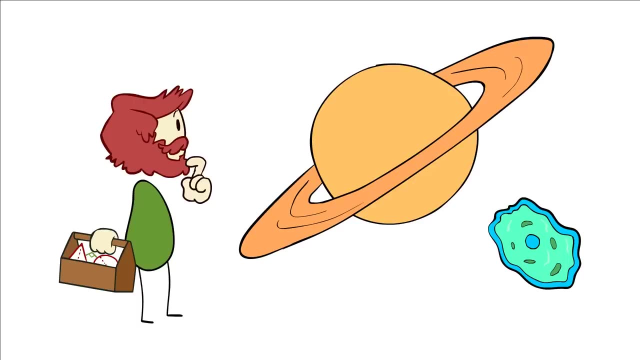 a way of reasoning that turned out to be profoundly valuable, but that only mimicked the real world on a very terrestrial scale. When we look at the vastly large or the imperceptibly small, we find that Euclidean geometry only offers us an approximation.